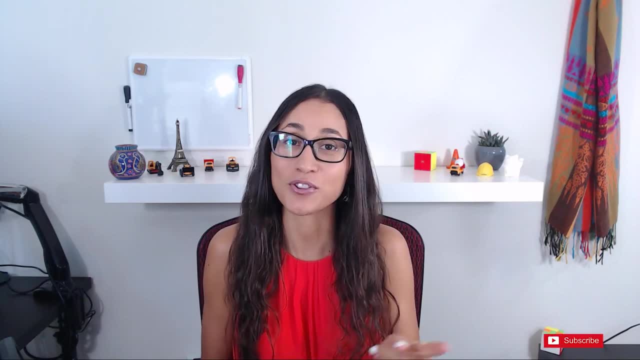 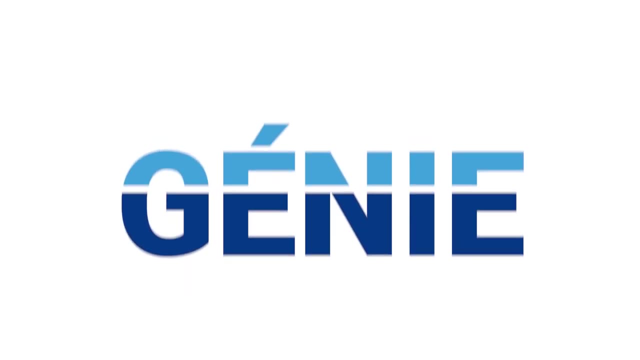 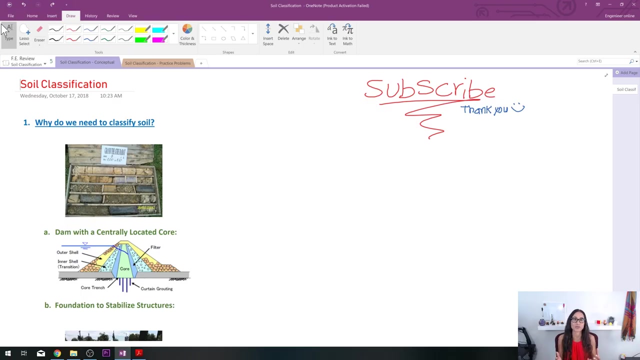 learn more about engineering, or just how to engineer your life better. don't forget to subscribe and make sure you hit the bell so you don't miss out on future videos. Now let's get started. The first thing we're going to talk about is: why do we need to classify soil? 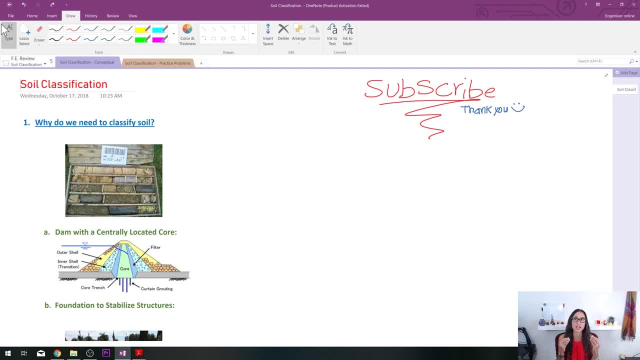 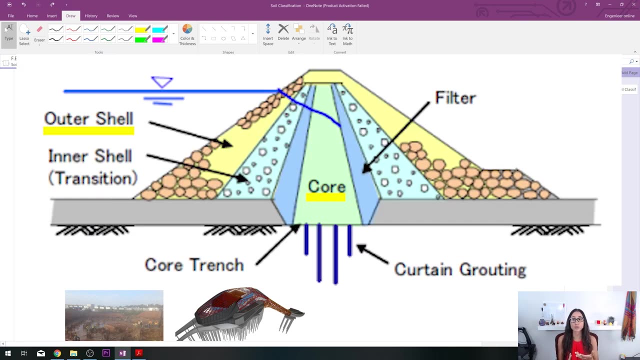 So in certain engineering applications it requires certain soil properties that we need for whatever system we're dealing with. So let's take a look at an example. So here we have a dam with the centrally located core right. So at the core. so we have two soils here that is applied to this system. So at the core we 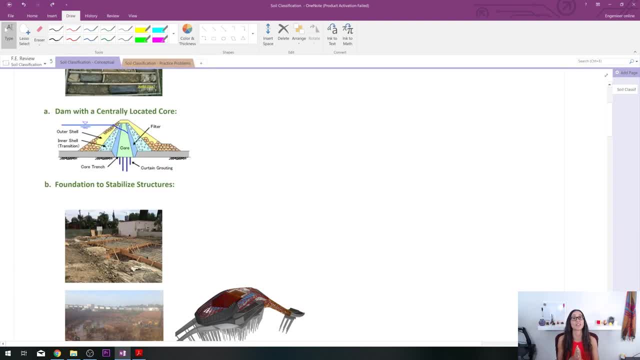 have a certain type of soil and at the outer shell we have a different type of soil. So at the core we usually use something like clay because, or a fine grained soil, and the reason that is is because we want water to be retained, and usually clay have those properties. 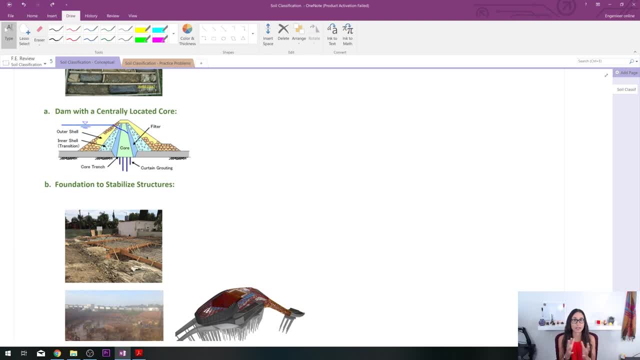 It's when there's water, clay usually expands, and so when it expands, it retains water. As for the outer shell, we need to stabilize the structure, so to do that, we actually need something more like grained soil, so more like gravel. So if we look at another example like 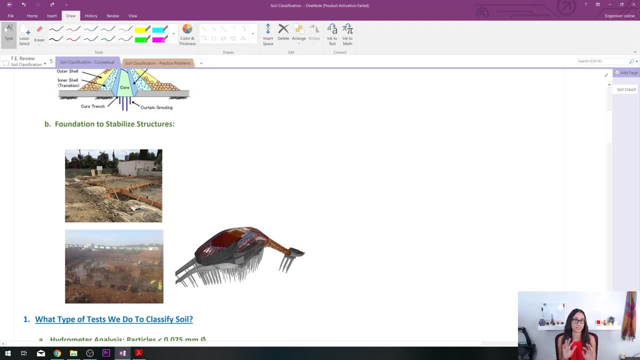 buildings, for example. we definitely don't want to build with clay, because clay can cause a lot of stability issues because it expands and shrinks. what it can actually cause is differential settlement. Let's take a look at an example here. So let's say we have a house here, right? 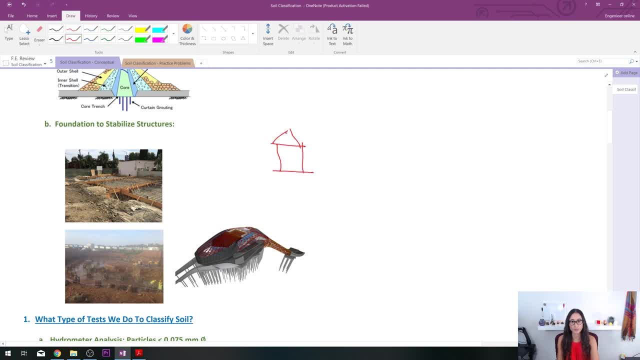 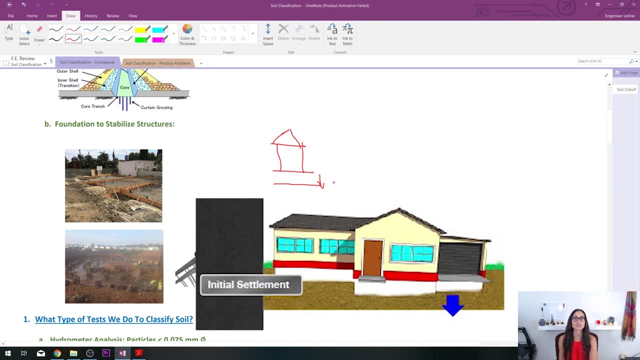 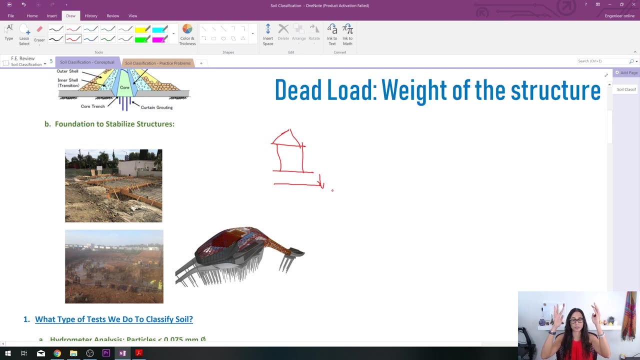 Let's pretend this is a house, So it's okay if this house settles uniformly, We have no problem. usually houses settle after construction. they settle a little bit because, like all, like the buildings, and the live load or the dead load kind of settles the house. Now what we don't want is 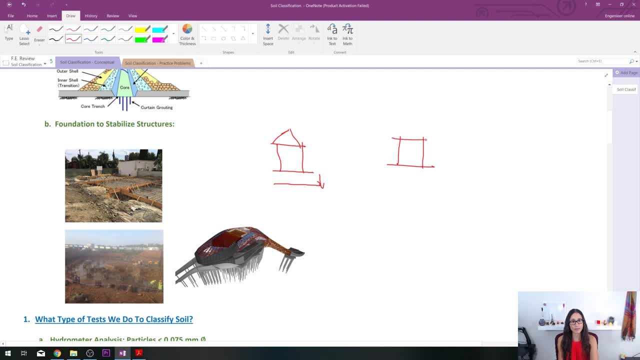 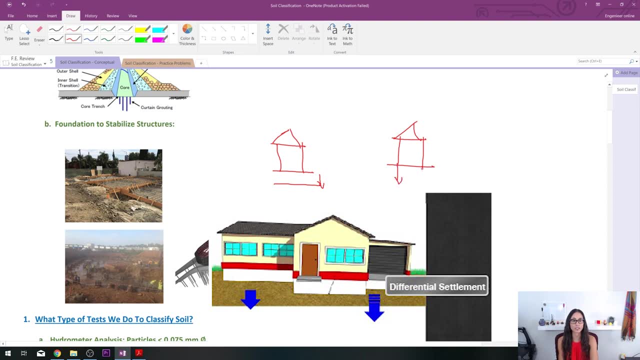 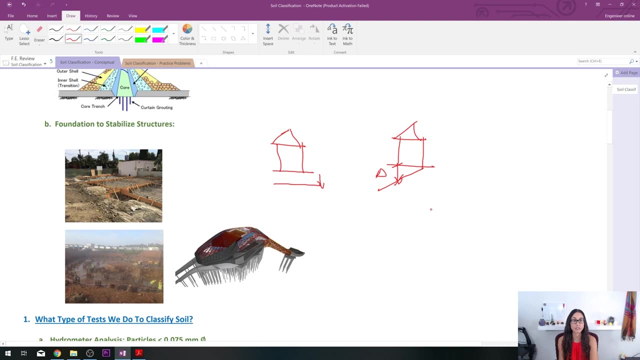 when a house settles at different like this side doesn't settle, it stays where it is, but then this side settles, it goes down right here and now. this is usually our settlement and that's what's called called differential settlement. So we don't want this to happen, because if the house settles so 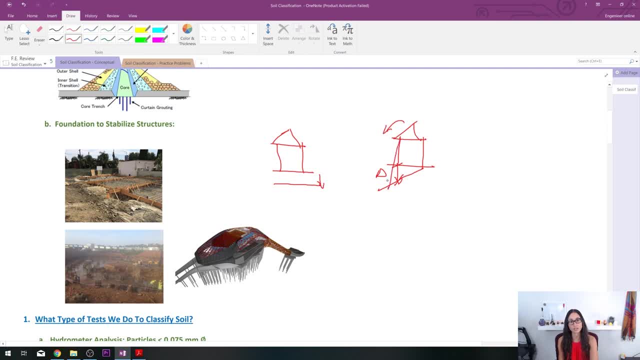 that means this moves, so this moves down all the way down because of the, the settlement and this right here stays where it is, and so that causes a lot of cracks in your house. If there's an earthquake, it's going to cause a lot more damage, so you don't want that, So that's why we try to. 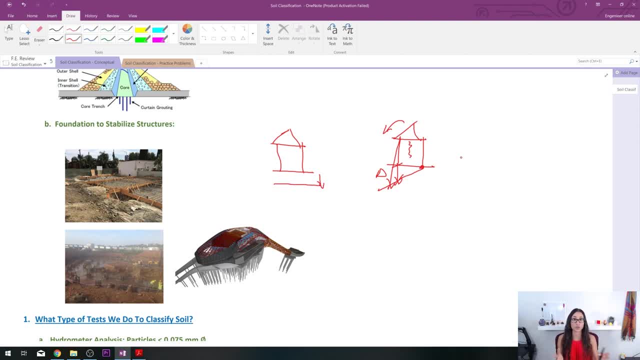 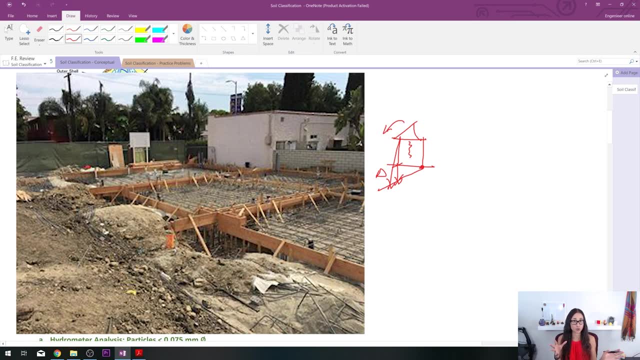 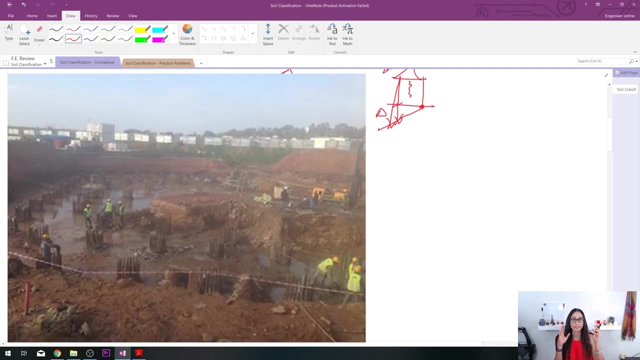 avoid clay during construction or when we're building. So here so this. this project had good soil, so the foundation was very simple. we just had like a continuous footing around the perimeter and then a four inch or five inch slab on grade. For the second project, however- this one, it had clay soil, the water table was high and it was. 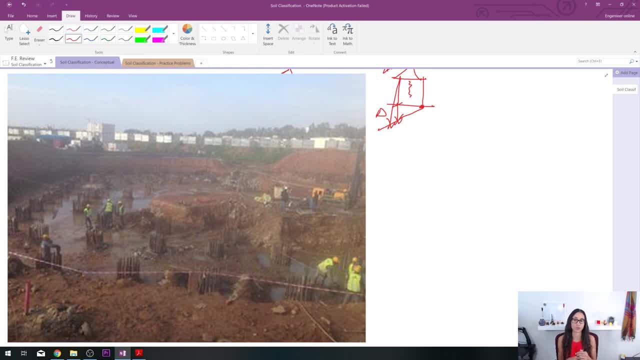 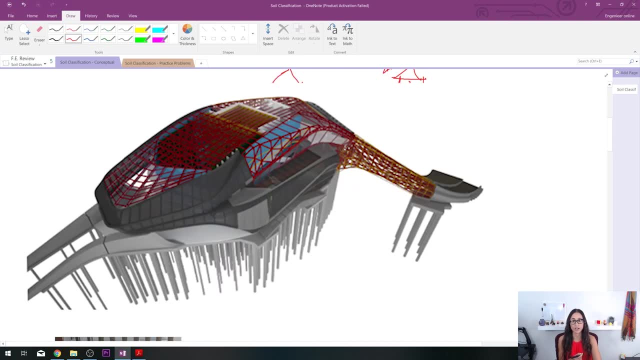 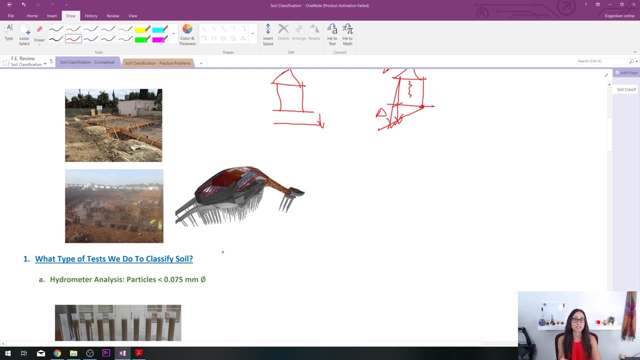 very contaminated water and really bad soil. So what we ended up doing is we had to build a lot of- as you can see, these are all piles right here around the building- to stabilize the building. So that's why it's important to know what type of soil we're dealing with, so that we can prevent. 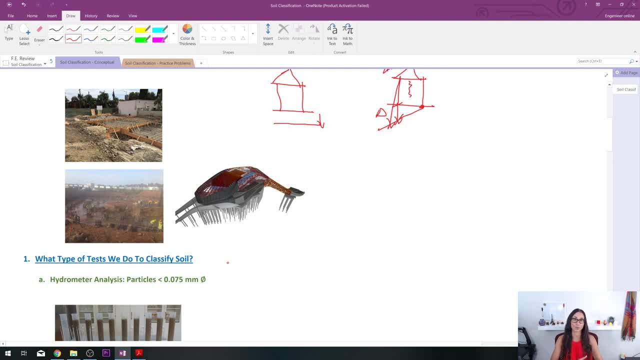 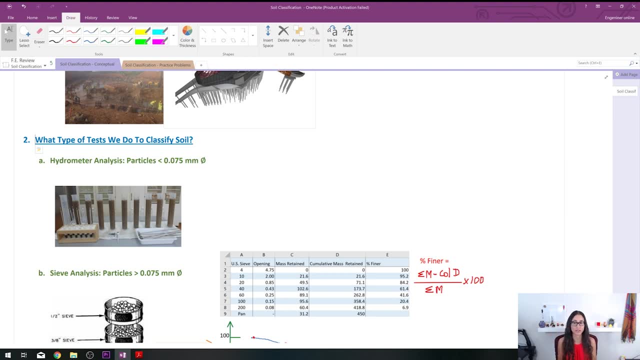 any damage to whatever system we're working with. Next, we're going to talk about the two tests to classify the soil. so we have hydrometer analysis and we have sieve analysis. Now this one. typically it's for particles that are less than 0.075 millimeters, and so what we do is: 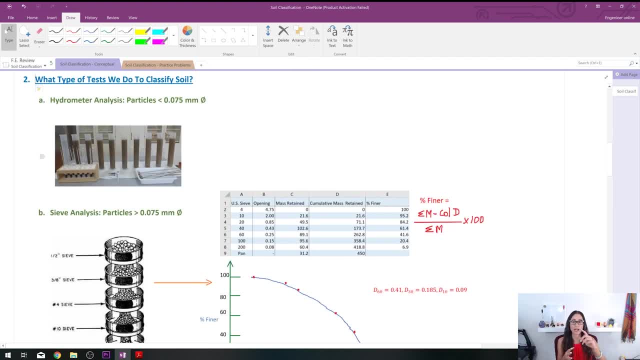 that we take soil, we add water and then we put the hydrometer bulb in it inside the the, the soil and the water, and then we take some recordings and there's some equations to uh to determine what type of soil that is. we're not going to talk about this too much because it's usually for particles. 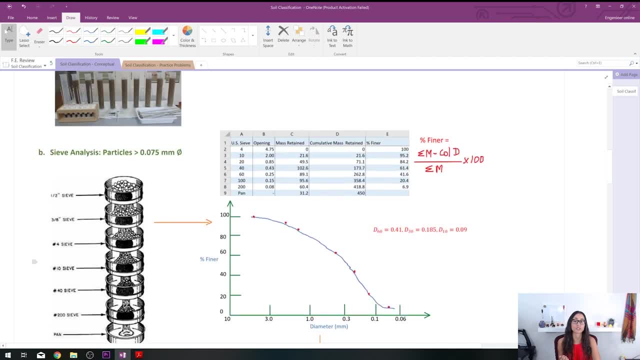 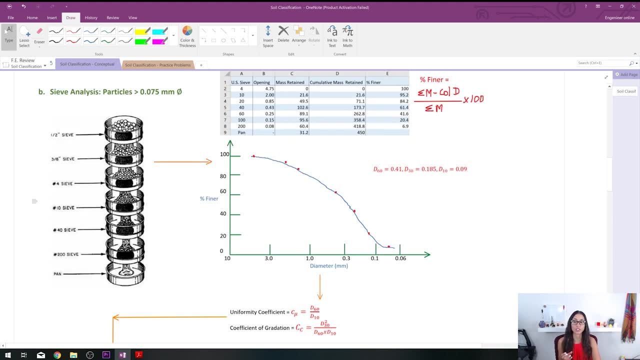 are less than 0.075. so mostly going to focus on the sieve analysis, which is for particles greater than 0.075 millimeters diameter. now, on here, we have different type of sieves that have different type of diameters, so and what you do is that you put the soil on top of the first seed and then you shake it till you get to the bottom. so the soil usually with diameters that, let's say, higher than 3, 8 inch, they would stay on the seed and if they're less, then they go down to the next one, and so on till you have what. 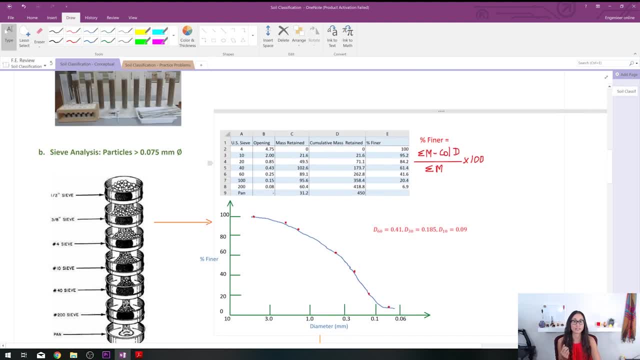 ever left in the pan. so once you do that, usually you get this type of data, you get: uh. so here you have the usc, which is number four, number 10, 20, 40, 60 and so on. these are the openings in millimeters. you have 4.75. that's the opening for each for the sieve, and then from the experiment you get the. 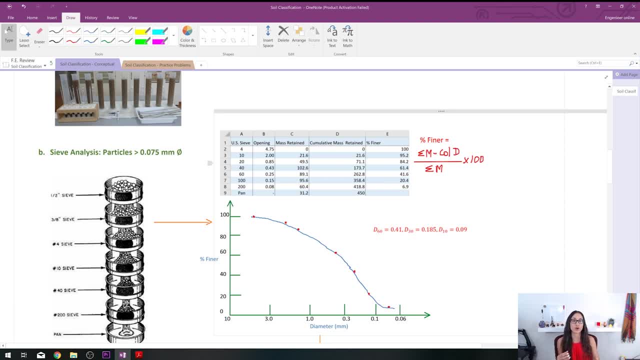 mass retained. so how much was it retained? or how much it stayed on that specific sieve? so, for example, on this one, on sieve number four, which is this one, zero, nothing stayed. everything went down, uh, to the next sieve. so then, at sieve number 10, we have 21.6, and so on. and keep in mind that these 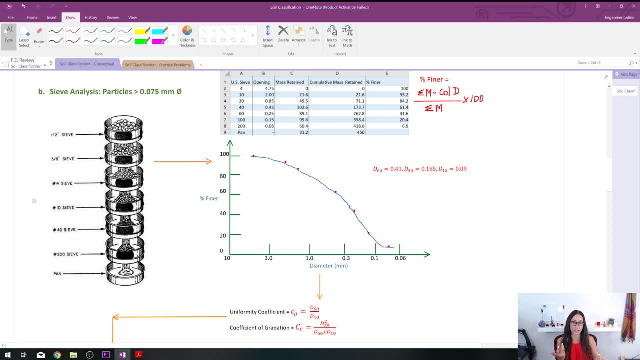 last years are usually silt and clay. they're fine grained and you and the more you go up, the higher you go up, or the more you have of these type of soils, then you have more like coarse grain. so once you determine the mass retained from your experiment, then you start doing. 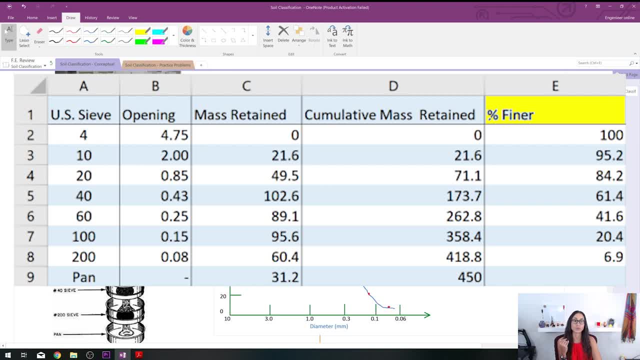 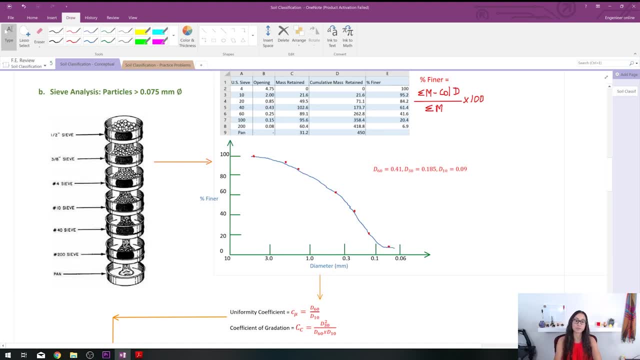 some calculations so you can get your percentage finer. the reason why we need to calculate the percent finer? because we want to get obtain a graph that is similar to this and from this graph we get two important uh variables, which is uniformity coefficient and coefficient of graduation. so we usually need these two coefficients so that we can classify the soil. 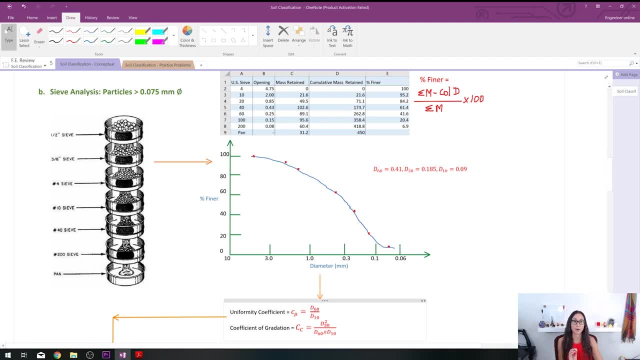 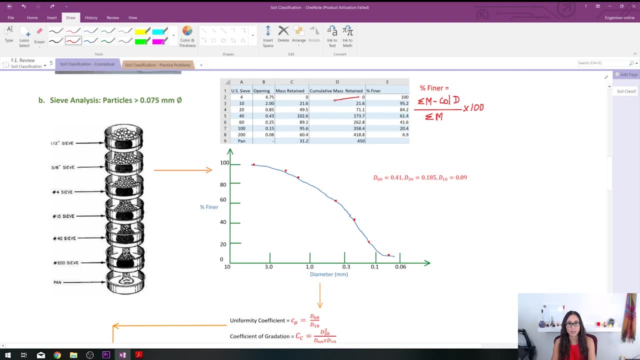 using the uscs, which we'll see in a little bit, so to calculate the cumulative mass retained. so what you do is you do zero and then you add it to plus 21.6 and that gives you 21.6. then you do 21.6 and then you add 49.5, and that's why it's it's cumulative. you're trying to add all. 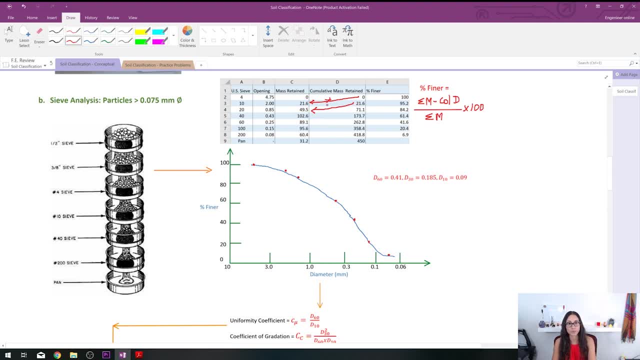 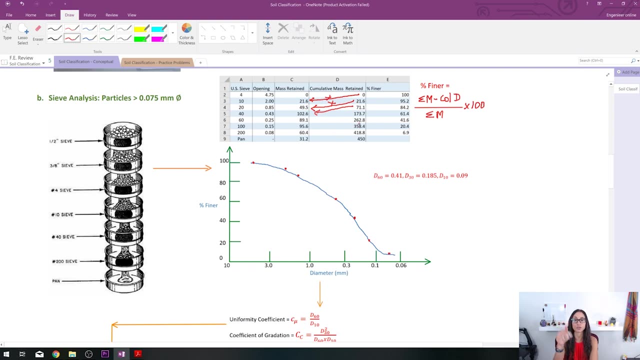 the mass retained. then you do um, so you add this 21.6 plus 49.5, that gives you 71.1. then you do 71.1, and then you add it to 102.2, six, which gives you 173.7. so you do the same thing throughout till the end. so at the end we 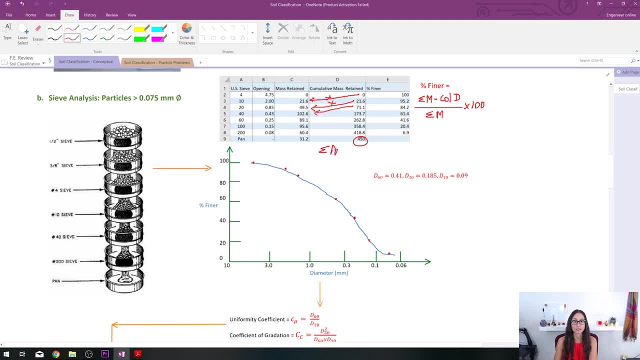 get 450, which is: this is your sum n. oops, so this is your sum m. right here, it's 450.. so then you calculate your percent finer, which is the sum m, which is 450 minus column d divided by 450, and you multiply that by 100, because we need a percentage. so let's take 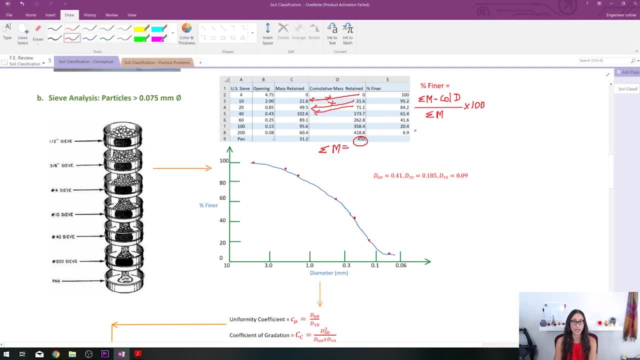 and the first one and do as an example together. so we have 450. that's my sum of n minus column d, which is zero. then i'm going to divide that by 450 and i'm going to multiply it by 100 and then this is going to give me this: cancels with this or the minus zeros, whatever. 450 divided by 450, just one. 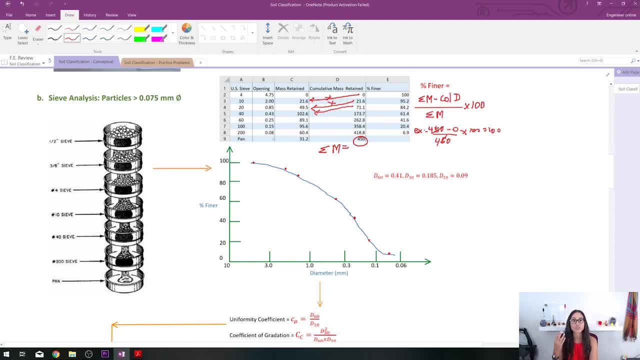 one times 100, you get 100. so that's exactly what i have. so percentage percent finer. uh, for sieve number four, i have 100, and then you do the same exact thing for the rest of them. once you get that, then you can graph pretty much what we do with. this graph represents. 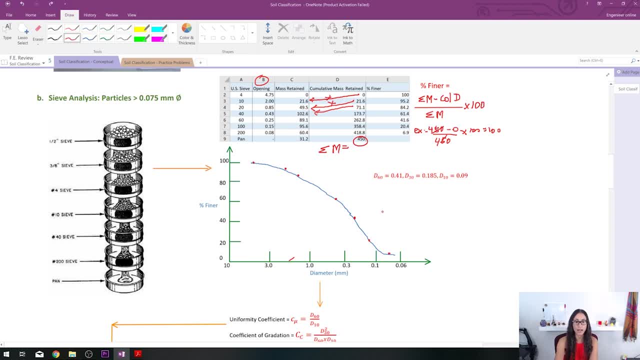 so this is b, that's here, that's b. and then, and this column e is graphed here. so once you do that, so i have 100. that's for sieve number four, opening 4.75 for approximately 4.75 is right here, and so that's where i have my point, right there, and you do the same thing throughout. 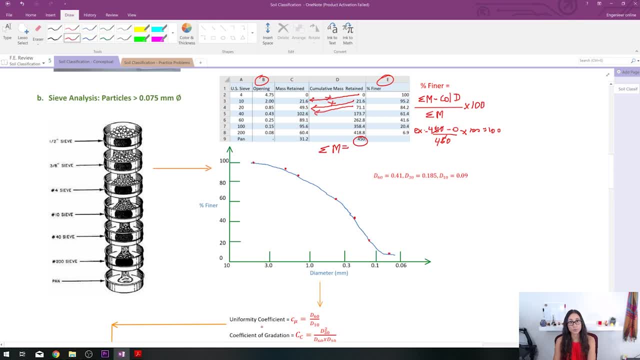 now to get the coefficient uh- uniformity and graduation- we need three variables from this graph. we need d60, d30 and d10, and i'm going to explain what these terms are exactly. so d60 is the diameter of the particle at 60 percent finer, and the same thing for d30 and d10. so 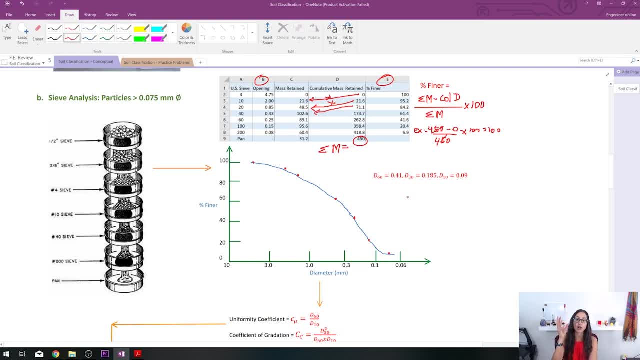 it's just the diameter of the particle at 30 percent finer. so let's, let's look at it together. so i have 60 here, right? so if i 60 finer, because i'm looking for d60, so i'm going to to kind of draw a line right here till i intersect my my graph. once i hit my graph, i have it right there. 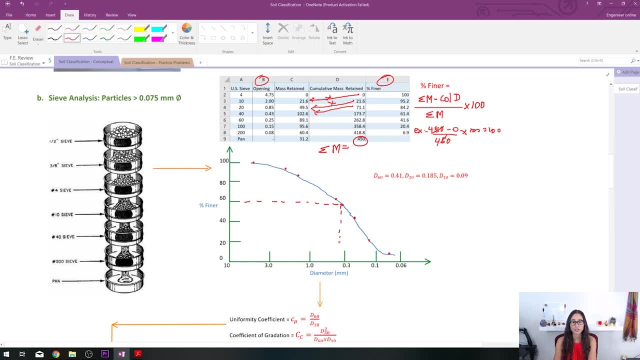 then i'm going to go down and i'm going to Parallels Line and tablespoons down and that gives me somewhere here which is approximately 0.41. then you do the same thing for d30- d30 is supposed to be somewhere here- 30 finer- and then you do the same thing. you 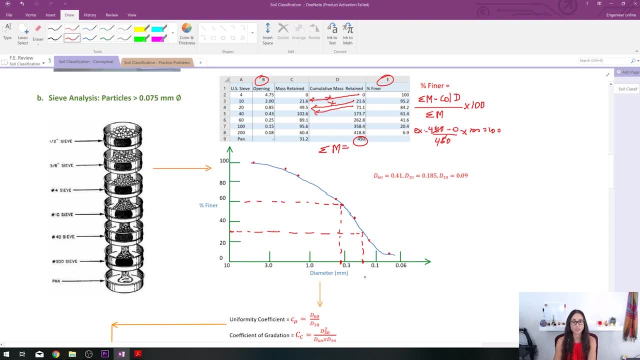 draw the lion and then you hit uh, you intersect your graph and then you come down so that you can find your diameter at 30 finer you about 0.185. and then same thing we do for d10, which gives you something about 0.09. so once you, 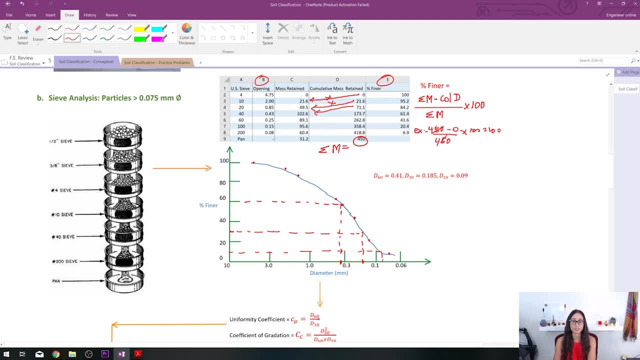 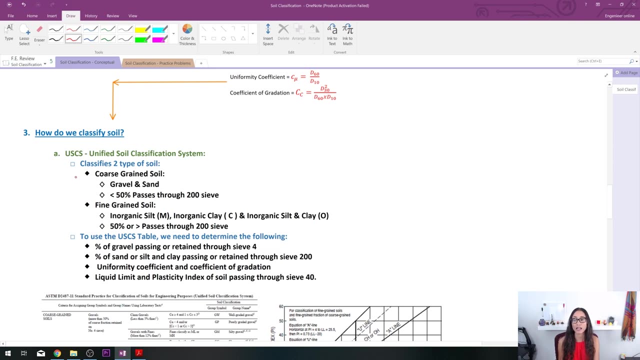 get that, then you can just plug it in here: you do d60, which is 0.41, and then you divide it by d10, which is 0.09, and then you do the same thing for cc. so now that we determine these coefficients, we will see how we can use this to classify soil using uscs. now, uscs stands for unified. 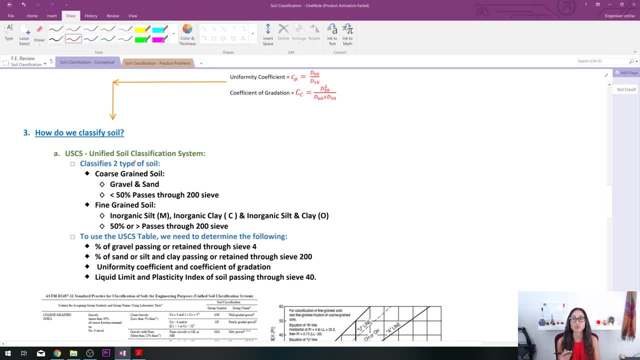 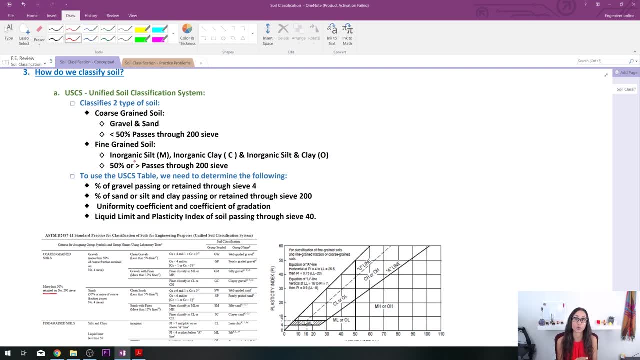 soil classification system and usually classifies two type of soil. we have coarse and fine-grained soil, like we talked about earlier, usually coarse. coarse grain is corresponds to either gravel or sand, and usually it's less than 50 percent that passes through the sieve, 200 meaning. 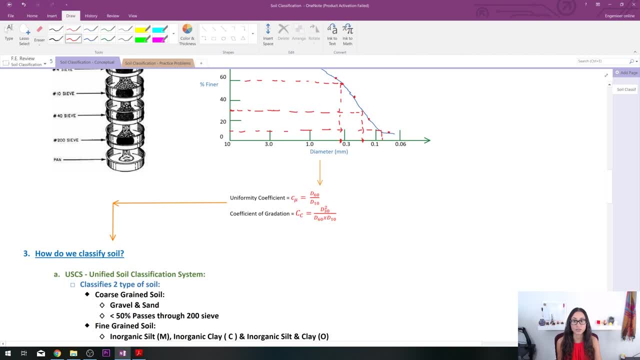 so if you take a look at this, we have the 200 sieve here. if you shake that 200 sieve and the particles that on there, less than 50% passes to, which means more than 50% stays on the sieve or retained, that means you have coarse. if you get 50 or more, that passes to. 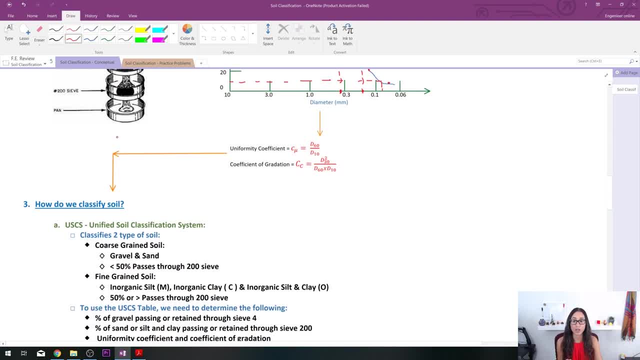 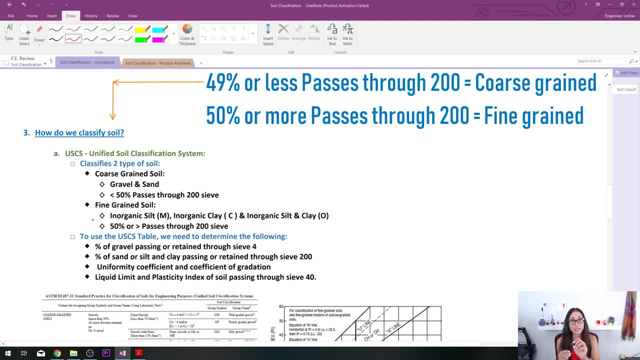 sieve number 200, that means you have fine grains. so remember, if you get the number 50 or more it's fine, if you get 49 that's gonna be coarse. but if you get 50 it's not coarse, it's fine grain. so be careful. you have to remember that a lot. 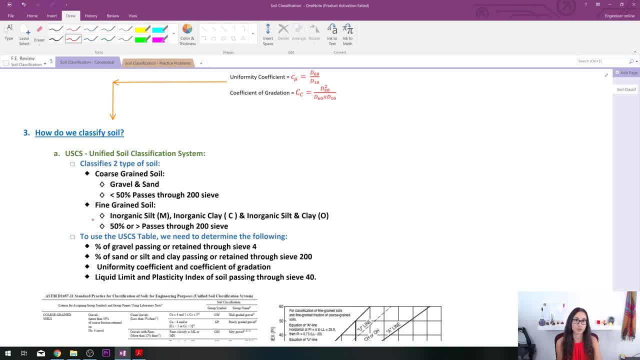 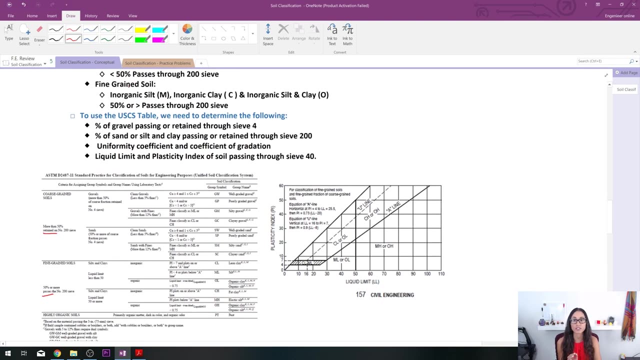 of people would think it's 50% and then they would just use coarse grain, which is wrong. so fine grain usually includes inorganic silt, inorganic clay or inorganic silt and clay. so once you determine these, or you have an understanding of the difference between fine grain and coarse grain, you can 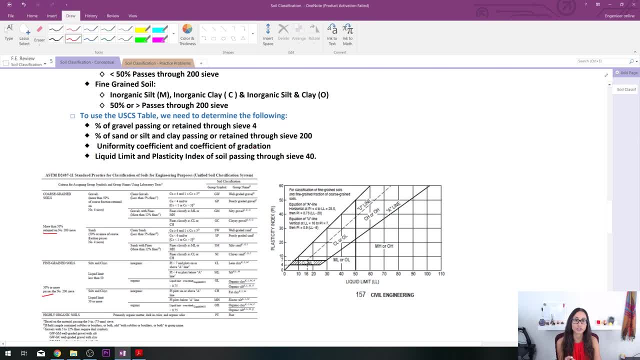 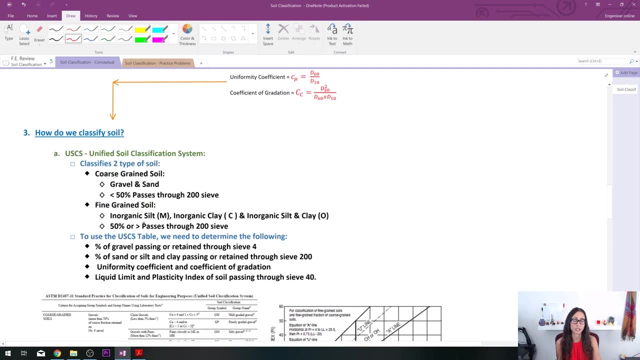 of these. then you need uniformity coefficient, coefficients of graduation, and liquid limit and plasticity index so that you can classify your soil. so here we have the table, so coarse grained. so remember- you don't need to really remember this because it's already on the table, but you have to understand it. 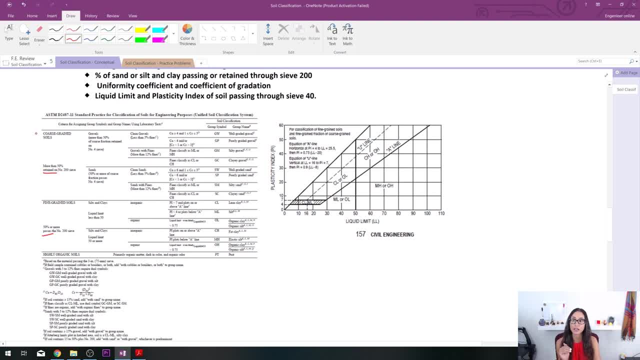 so that you know how to use the table. so this is really important. so here we have coarse grain. this is more than 50%. note here that they use the term retained and not passes, so be careful with this. here, however, they use the term passes, so this can be a little bit tricky, especially under an exam, and 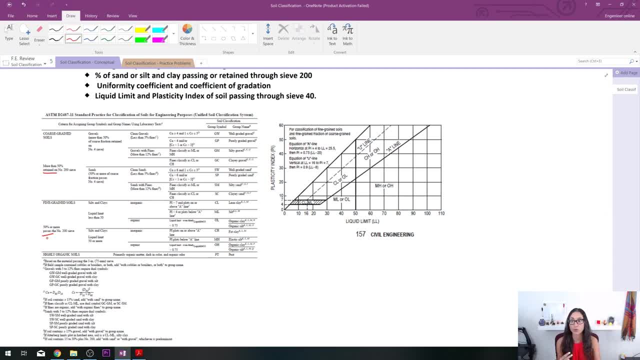 then the pressure. so make sure you differentiate between the two. this more than 50% retained, it just really means less than 50% passes to receive 200. so it's the same exact thing here. as you can see, it says 50% or more passes to. 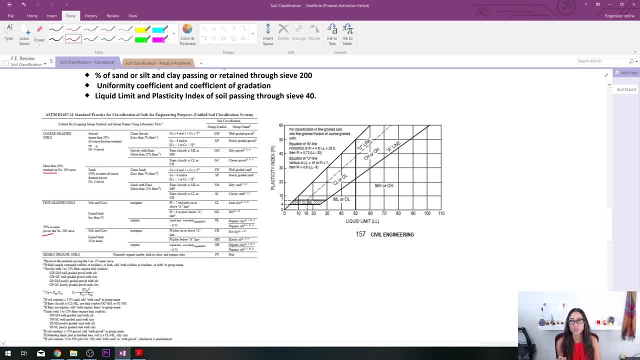 the 200, and this is defined as fine grain and coarse grain. so let's take a look grain, once you determine the gravel, or if it's sand and so on. you get on here and this is when you start using your coefficient of uniformity and gradation and the liquid limit and plastic plasticity index. so this is why 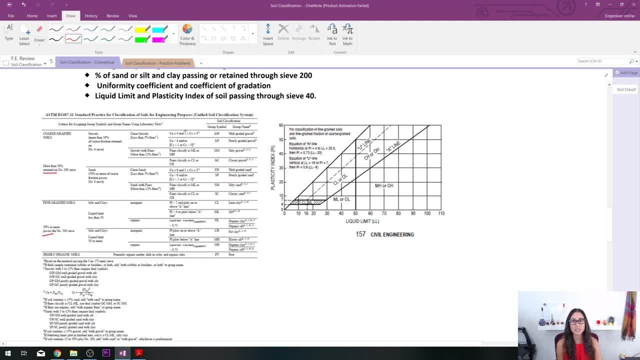 it's important to know those terms. when we'll do more problems this, these terms will become more clear. I also want to cover a little bit of the terms, so make sure you know what these really stand for, because it just helps you understand, have a better understanding of the soil. so G just gravel, S is sand, C is clay, M. 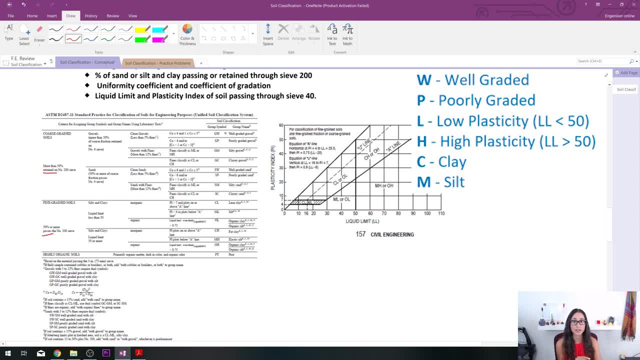 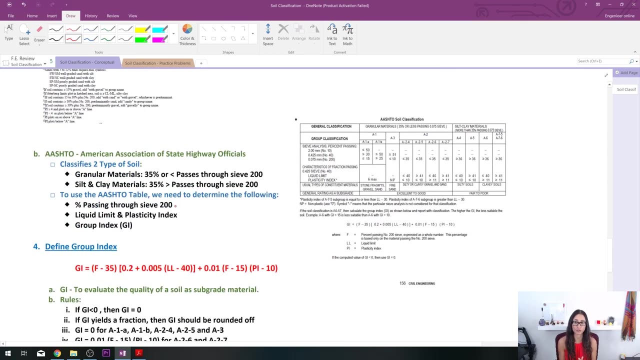 is silt and O is just organic clay and silt. now for W is well graded, P is poor graded and then I think I think we covered all of it. that is all for all USCS. so for AASHTO, American Association of State Highway Officials, usually, 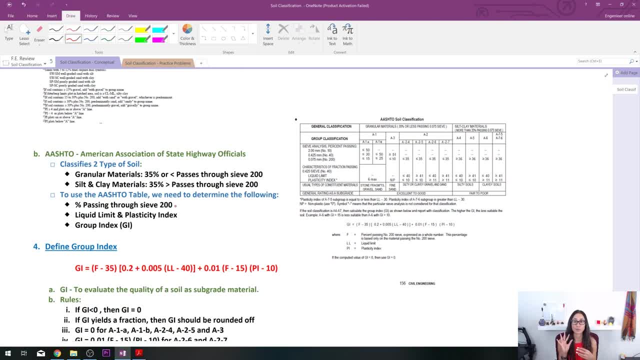 classifies the same type of soils. so we have 35 percent or less passes to sieve 200 and that is classified as granular. as for if it's 35 percent or more passes to sieve 200, then we have silt and clay. now we 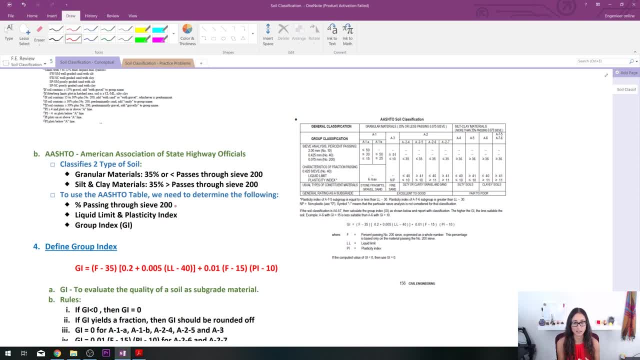 also need to determine liquid limit and plasticity index, just as we did for you, SES. but on top of that, we need this term group index, which is GI, which is something we're going to talk in a little bit, but before we do that, I want to go over the table now. the table is: 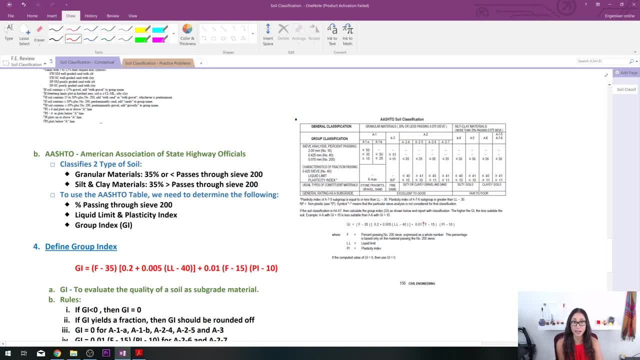 this. i got it from again the same thing, the ncs handbook, and it's on page 156. so, um, this is the it tells you here. this is granular material which is 35 or less passing to sieve 200. this is 0.075, is just um, if you guys remember, that's the opening in millimeters and the same. 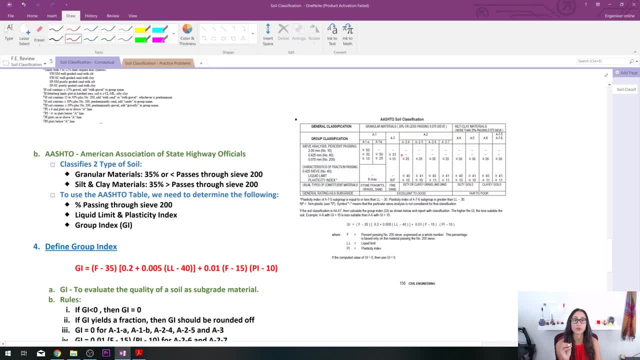 thing: here it tells you more than 35. now remember, if you get 35, exactly 35, you gotta classify that as granular material, not silt clay, because here it says 35 or less. but then on silt clay it says it has to be more than 35. that means anything greater than 36 goes under here, anything 35 or 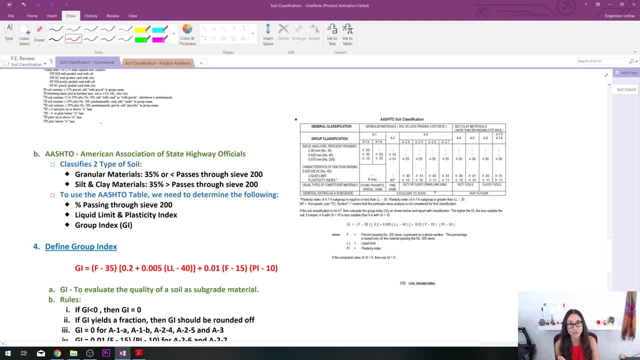 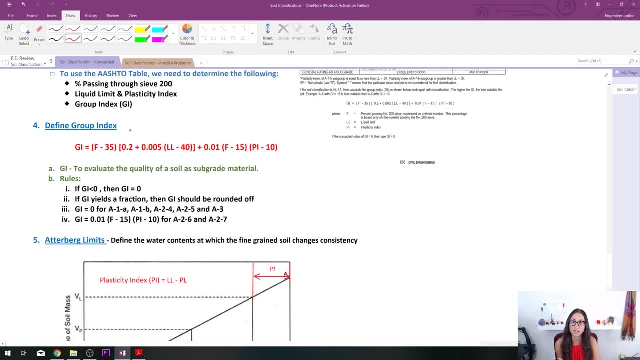 less goes uh class if it gets classified under these groups. so, keeping that in mind, okay, so let's talk about the group index. so, group index: this is the equation we have. this first term usually, um, it defines the liquid limit and then, in this equation, it defines: 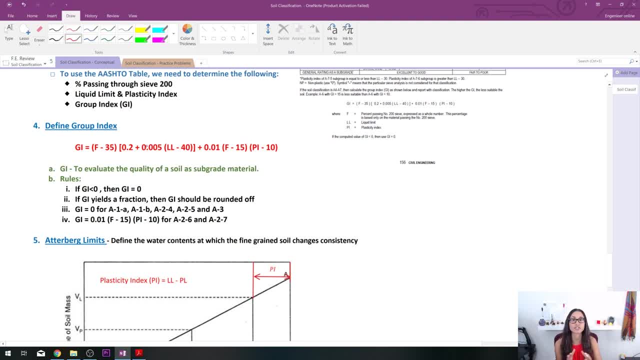 the plasticity index. so gi is just a way to evaluate the quality of the subgrade material, usually for highways. so there's certain rules that you need to keep in mind for gi. some of them are covered here and some of them you just have to try to remember them during if you're going to take your fe. so ge if gi is negative or less than 0. 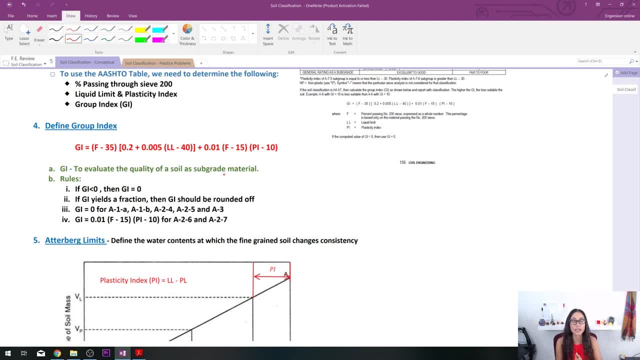 then you just assume it equals to zero. if ge yields a fraction, which means like if it's 2.2, you just round it up to four. triangular is equal to zero for certain for these types of groups: a1a, A1A, A1B, A2-4,, A2-5, and A3.. And GI is equal to this part of the equation for A2-6 and A2-7..